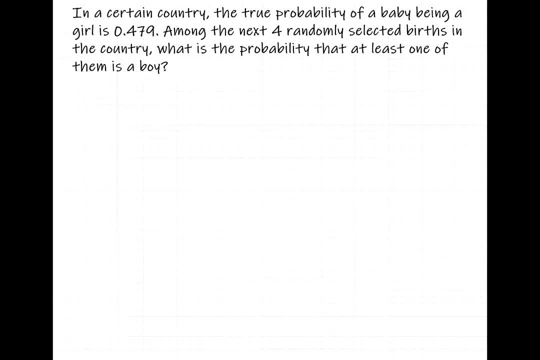 All right. so this, at least at first glance, this seems like a situation where we want to use the complement's rule of probability, and the reason we want to use the complement's rule is so: among the next four randomly selected births, 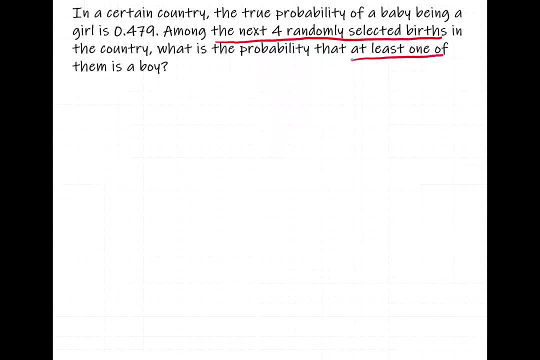 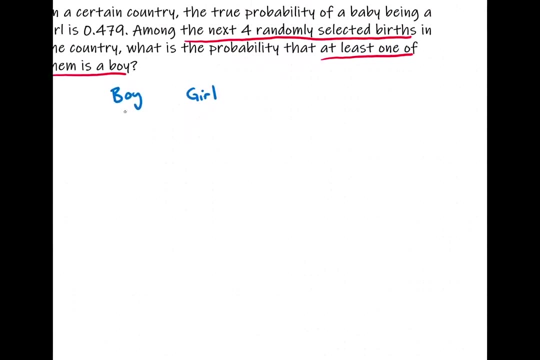 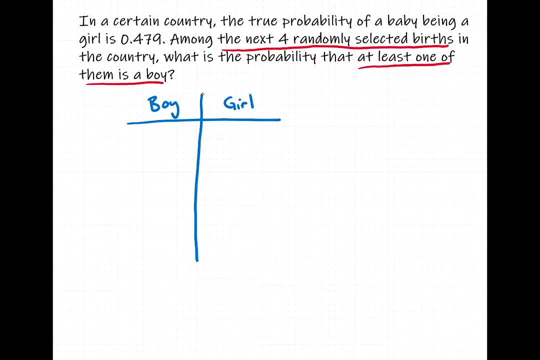 we need at least one of them to be a boy. Now, at least one means one or more, so let's say that one of them is a boy. Let's look at the possible scenarios. Let's say boy and girl. So if there's four kids, you could have all girls. 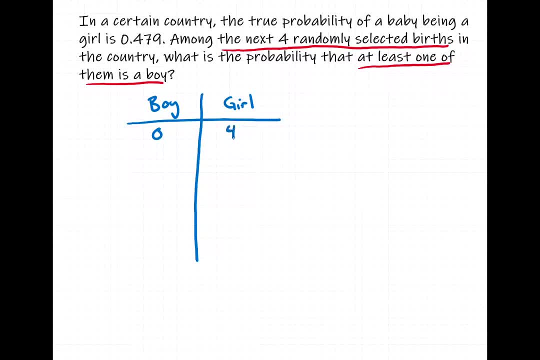 So zero boys and four girls. That's one possible scenario. Or you could have one boy and three girls, You could have two boys and two girls, You could have three boys and one girl, Or you could have all four boys. So these are the possible scenarios. 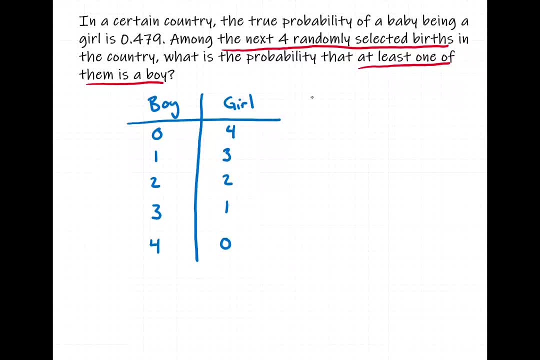 And what we're looking for. we want the probability. So actually, this is, before we talk about probability, The event that we're looking at, we'll call this event. A is at least one boy. Now, at least one boy means, like I said, one or more boys. 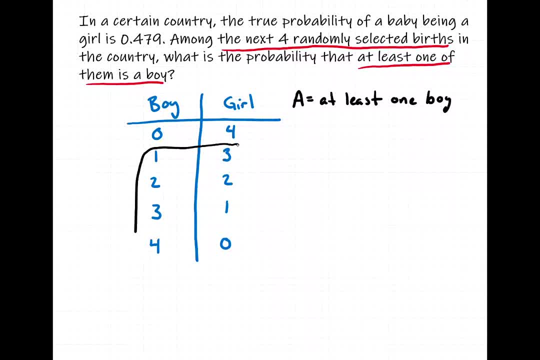 So that is referring to all four of these scenarios, all four of these cases. So that's our event: at least one boy. So it could be one boy, could be two, could be three, or it could be four And the complement. so let's do a different color here. 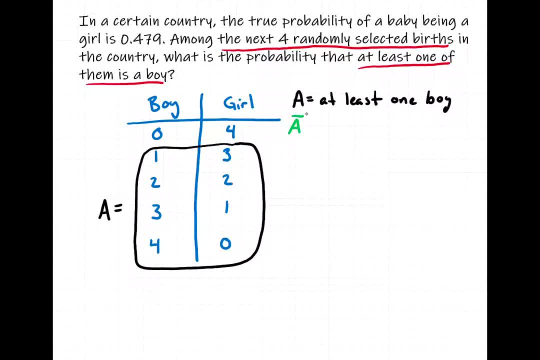 The complement of this event. If it's not at least one boy, the complement would be no boys, And so the complement could only happen one way: zero boys and four girls. So this would be the complement of our event, And since there's many different ways, 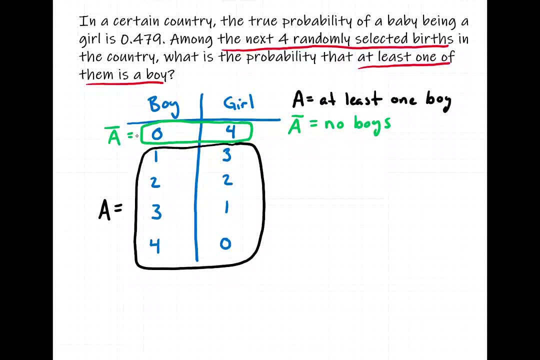 that at least one boy could happen. but there's only one way that the complement of that no boys could happen. We could use the complement's rule of probability, which says the probability of something happening is always equal to one minus the probability of that thing not. 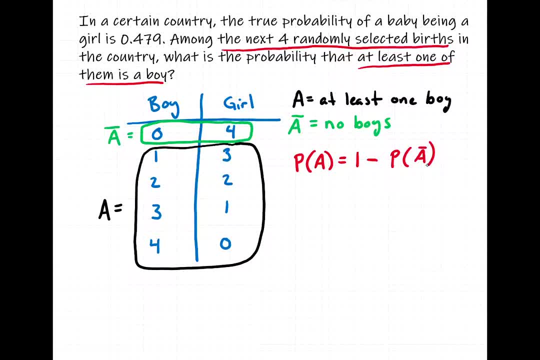 happening. And so let's see if we could calculate the probability of the event A not happening, the complement of event A, And so this would be. so this right here would be four girls, excuse me. So that's four girls, zero boys. 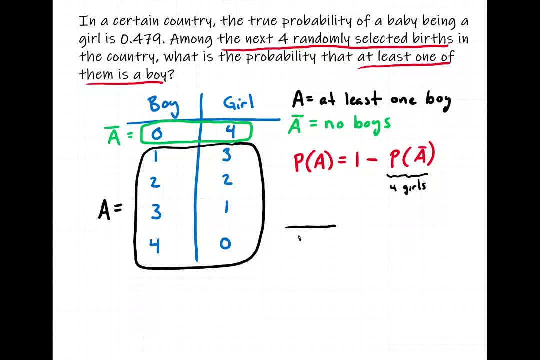 All right. well, if we look at child number one, what's the probability that first child is a girl? Well, we know that's given in the problem. That's 0.479.. And Girl number two, What's the probability of? or child number two? 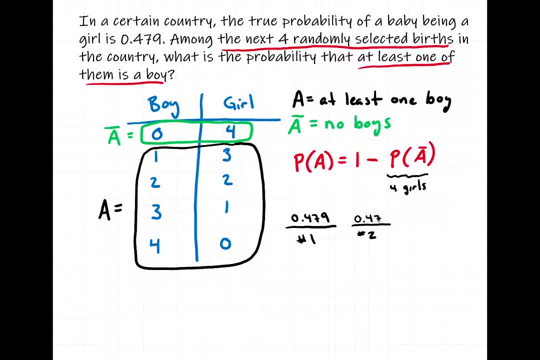 the probability that child number two is a girl is also 0.479.. And child number three being a girl: 0.479.. And finally, child number four being a girl: 0.479.. So four girls means the first one's a girl. 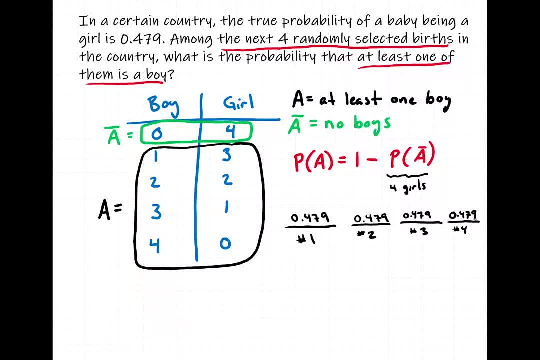 and the second's a girl, and the third is a girl and the fourth is a girl. Remember, and means multiply. The multiplication rule is the rule for, and So we're going to multiply these four numbers. So that means the probability of our event A, which. 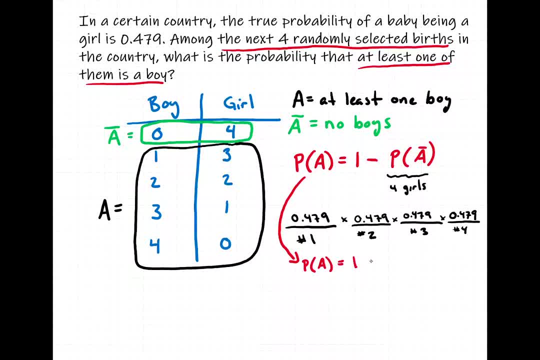 is at least one boy is equal to one, minus the probability of no boys, which is 0.469.. OK, four, seven, nine times, itself four times, or we could say to the fourth power: all right, and that should do it for this problem. now we just have to crank out the number.